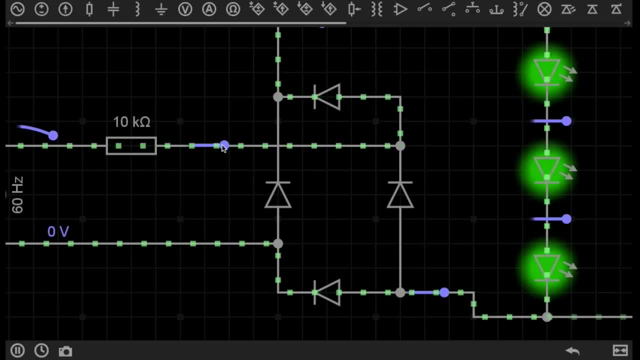 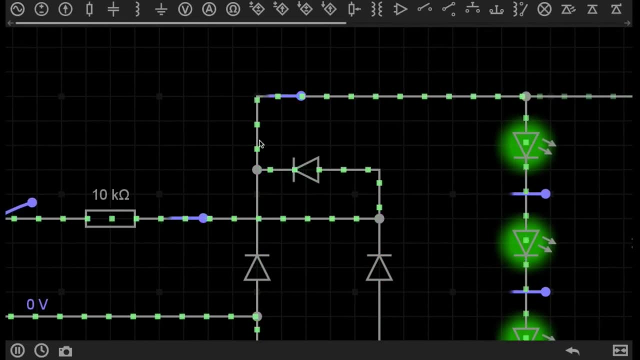 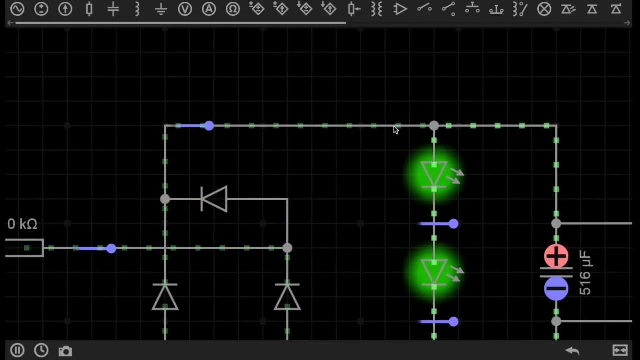 basically make the alternating current flow through all of these diodes in a way that when the electrons actually flow out to the rest of the circuit, they're always flowing in one direction. But you can see they are not alternating back and forth, they are simply. 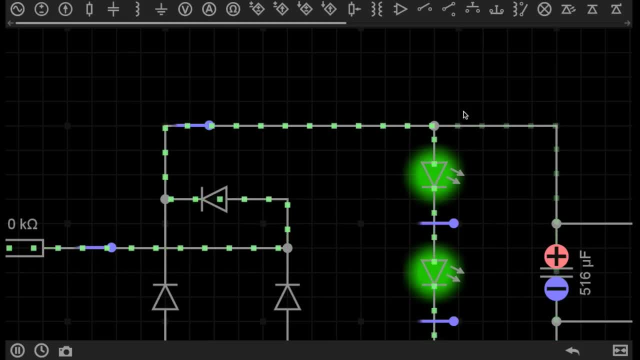 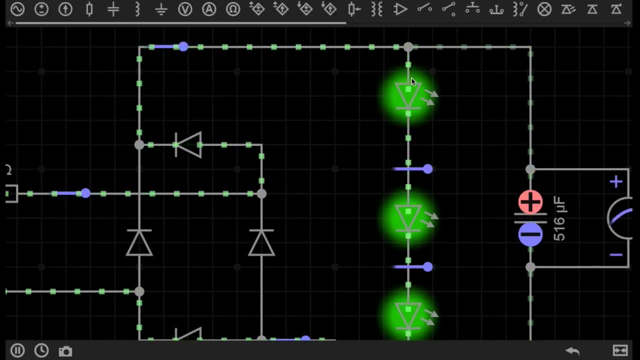 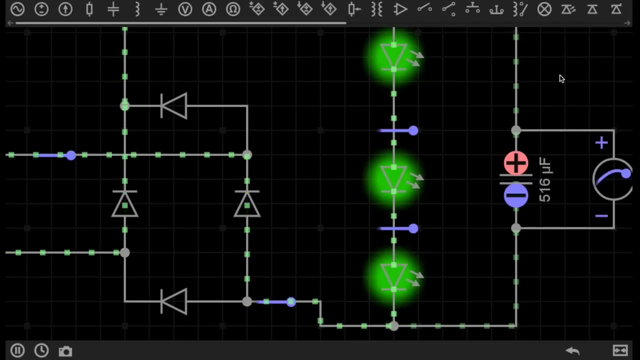 going straight forward in one direction, with very small pauses as the AC supply hits zero on the wave, And so that means I can power these LEDs, Because if they were actually being powered from alternating current, these LEDs would be flashing and would look absolutely horrendous. Now the easiest way to see the current is to use the LED. 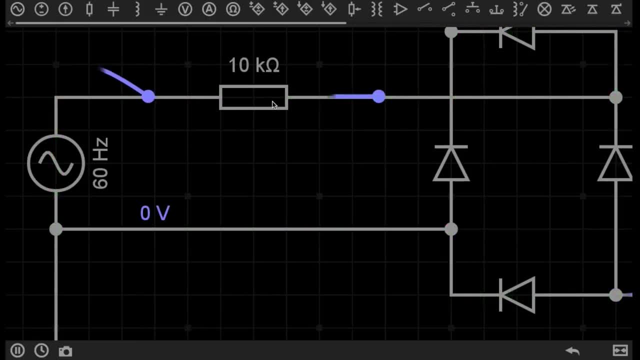 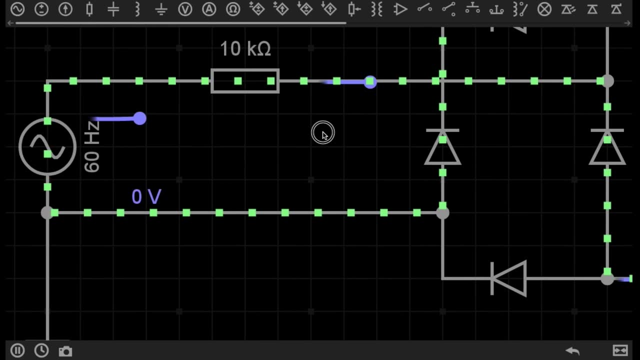 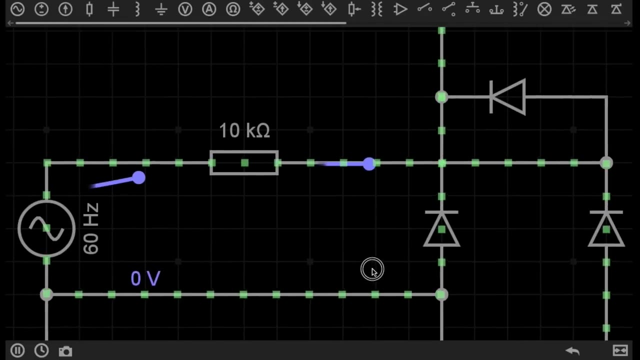 So I'm going to slow this down even more so we can follow the electrons even easier. We can actually follow the electrons on each part of the wave to see what's happening, As the electrons are now about to move the other way. watch what happens. So here we go, the electrons will start moving this way. 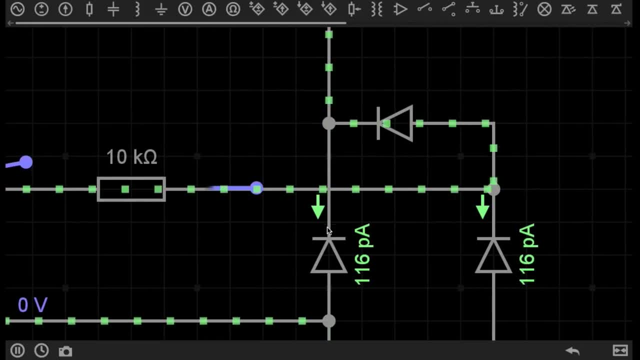 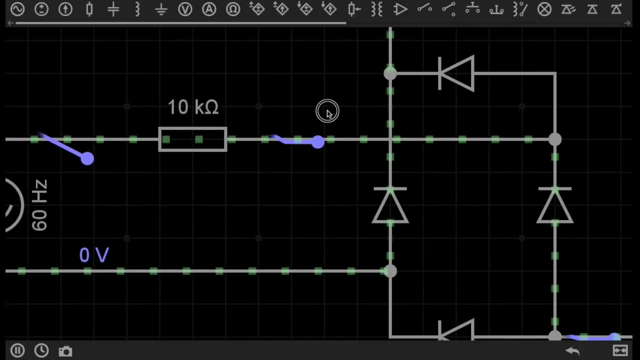 and it won't pass through this diode, because this diode is in the direction which will not allow current to flow. So instead, the current now flows through here and through this diode, pushing all the electrons up here, And as the current starts to change, now you can see that it's flowing through this diode. 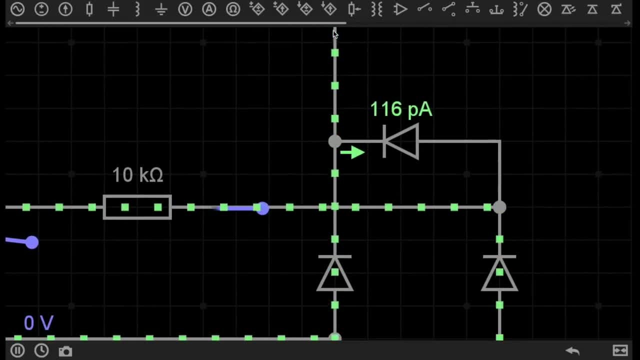 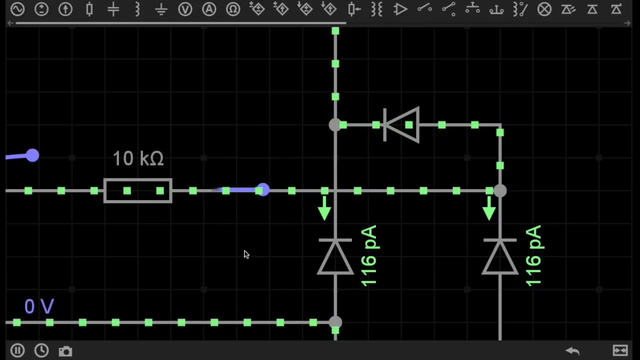 and again going up in this direction. So that means on each high of the AC wave the electrons are being pushed in that one direction, because only one diode here will allow current to flow on each alternating wave, And the same happens on the returning end. 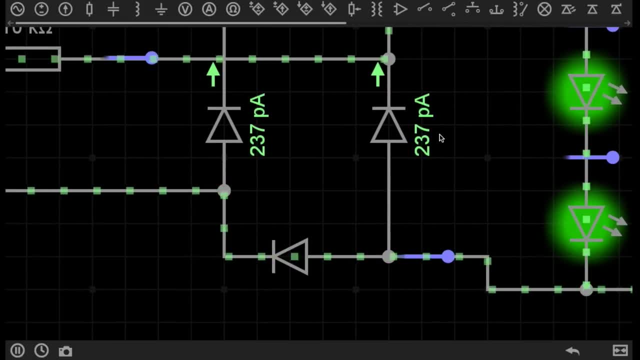 as well. So we've followed it from this side, and there are another two diodes to obviously complete the circuit, which means that when current flows backwards this way, it goes all the way up here round to the LEDs, and then it goes back this way, So you can see that the current is being pushed in this direction.